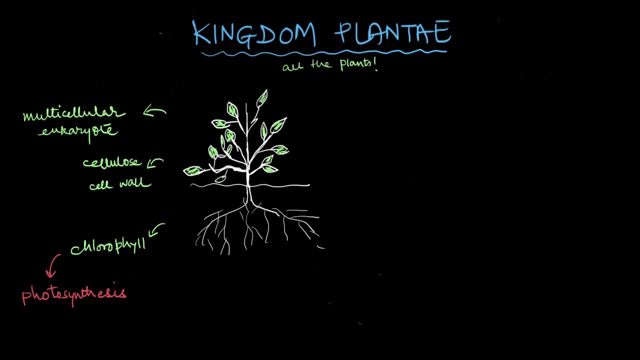 You know the process by which plants make their own food, And all plants have chlorophylls A and B for this purpose. That means all plants are autotrophic. However, some plants also seek nutrition from other organisms, Like the Venus flytrap, for example. It traps insects. 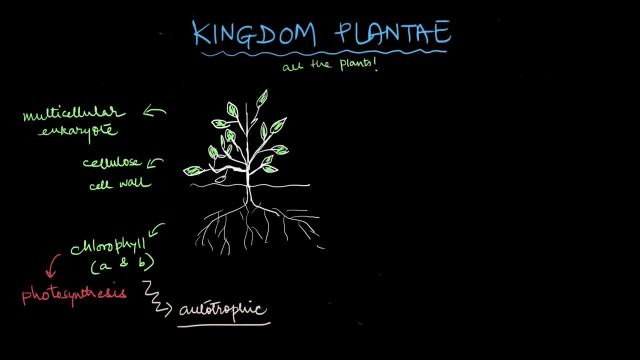 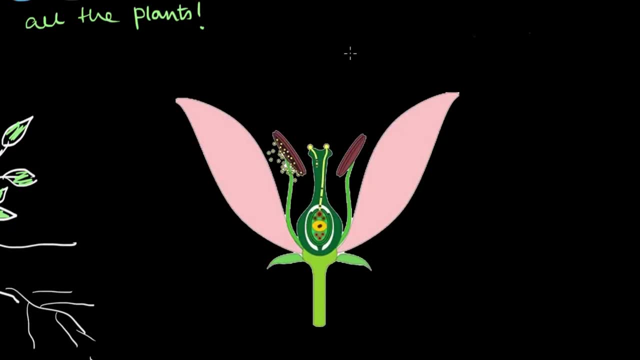 and consumes them for nutrition. Yet another characteristic thing about plants is that they are complex reproductive structures. Take a look at this picture right over here. This is a flower of the hibiscus plant, and inside this flower you will find the reproductive structures of the plant. Now, these structures, they are multicellular containers where they 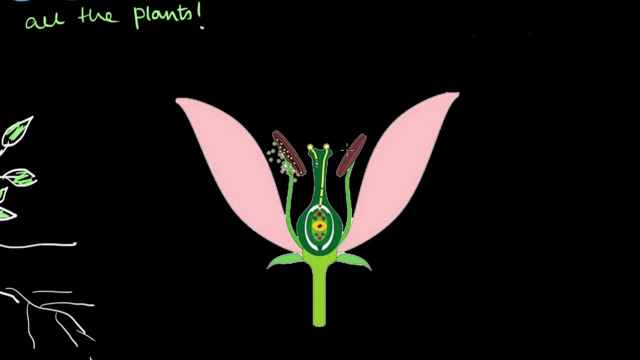 are kind of like multicellular containers where the gametes are produced or they are formed. Now, this one right over here, this is the male reproductive structure which is going to produce the smaller motile male gametes. And the one right in the middle, this part, this is the female reproductive structure. 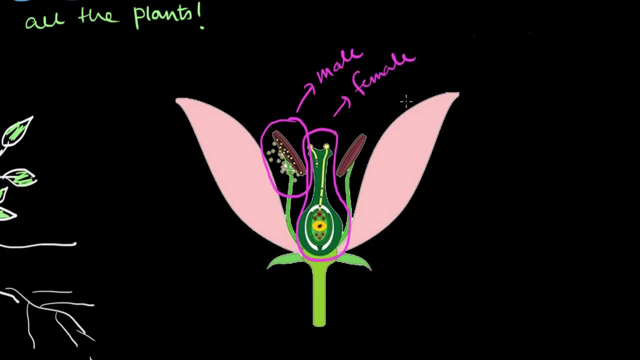 which is going to produce the much larger non-motile egg or the female gamete. The gametes will then fuse together to form a zygote, which will eventually give rise to a new plant. Now the female reproductive structure is made in such a way, or it has evolved in such 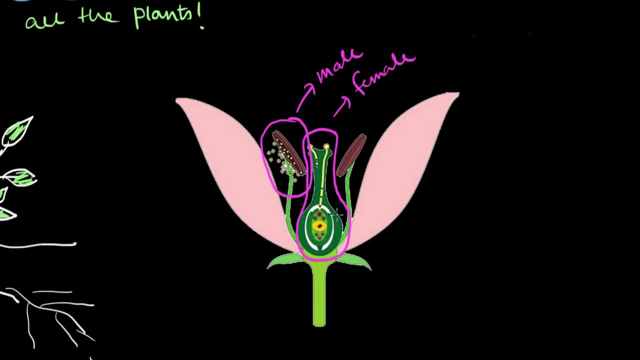 a way that it is equipped to provide nutrition to the embryo as well. Such a level of complexity is not something that you will find anywhere- other organisms like protists or fungi or any of the members of the kingdoms which come before plantae. So this is a kind of complexity that has evolved from plants onwards and it continues to become. 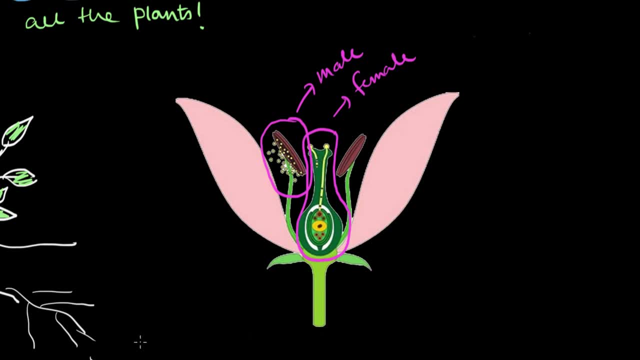 more complicated as we move on to the other kingdoms, which means the kingdoms that come after plantae, by the way, like animals, for example. Oh, and these extra structures that you can see which are surrounding these reproductive structures. they are composed of normal cells, or rather non-reproductive cells. 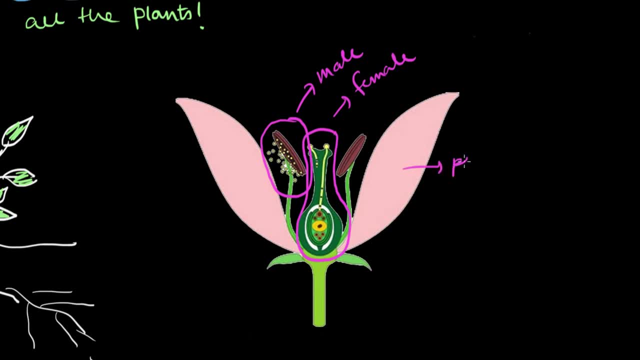 So the cells which you will find in this petal right over here or in this sepal right over here- So this is a sepal- The cells you will find in either of these structures, they are not going to be reproductive in nature, but they will be non-reproductive cells, and that's why we say that these complex 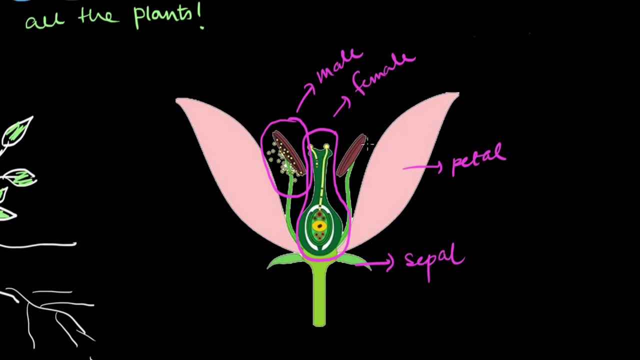 reproductive structures. they are surrounded by non-reproductive cells. So this is what we mean by it, Because the petals and the sepals which are surrounding them, they are not made of gametes. You won't find any kind of reproductive cells in these structures. 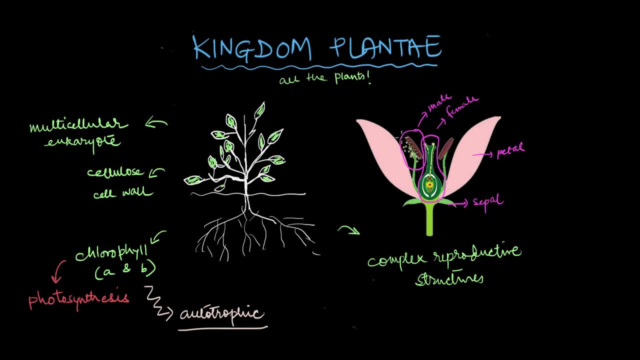 Now there are more plant characteristics to explore, but those are more specific to a certain type of plant. So let's take a look at the different types of plants that you will find in the plant kingdom, Based on certain things like body parts, specialized tissues and seed production. all plants have 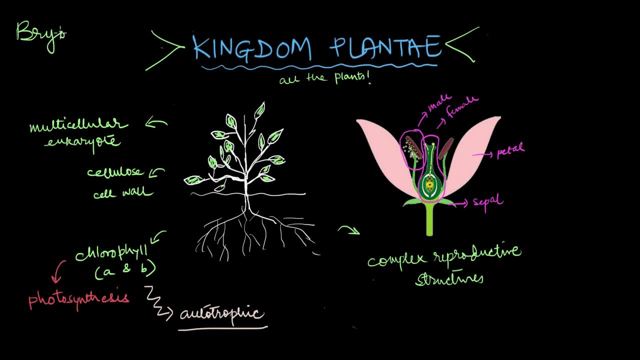 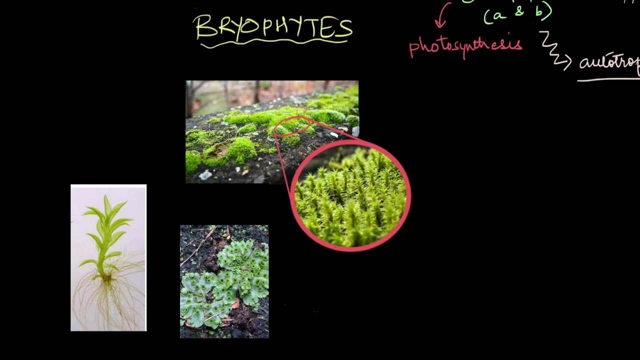 been categorized as non-reproductive. They are categorized into four divisions: the bryophytes, the pteridophytes, the gymnosperms and the angiosperms. Let's check them out one by one. Starting off, we have the simplest members of the plant kingdom, the bryophytes, or division. 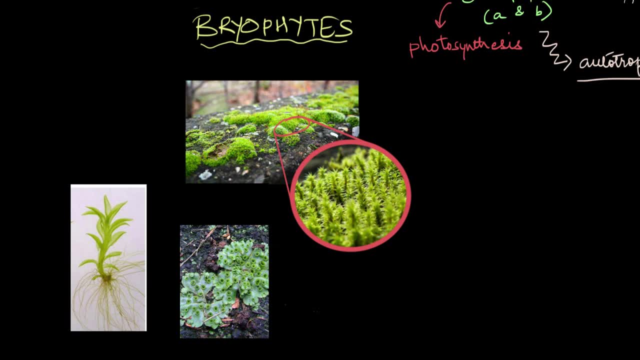 bryophyta, which includes plants like mosses, liverworts and hornworts. Bryophytes are seedless, comparatively smaller plants whose bodies are unorganized. There are some bryophytes which show root-like, stem-like or leaf-like structures, kind of 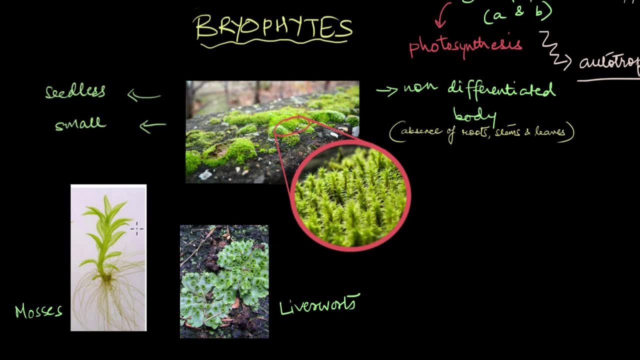 like this. And then there are some bryophytes which have this simple plant body which is kind of like a huge accumulation of cells, like a huge blob of cells, you can say, And it's just one plant body which is called the thallus. 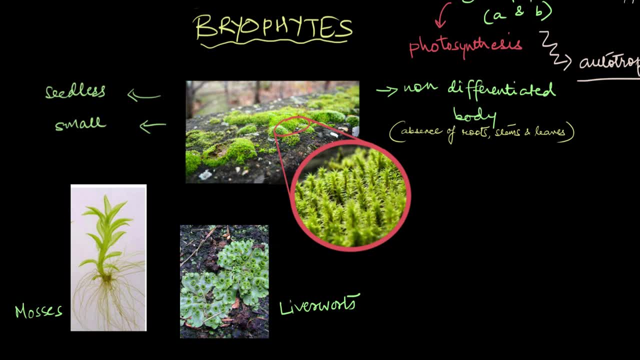 Kind of like how we call it, How you can see in the liverwort over here, And this entire plant body or this thallus is attached to the substratum or the ground with the help of these thread-like structures called rhizoids, something you can see here. 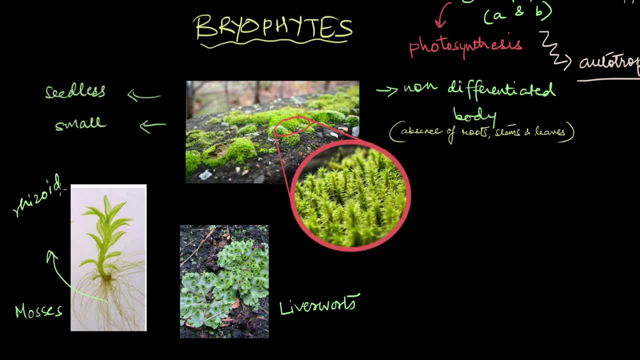 in this moss too. So these are rhizoids, which are root-like structures. Now, they may look like roots, but they are not actually roots. That's what I mean by root-like or stem-like or leaf-like structures. they are not exactly the real deal. 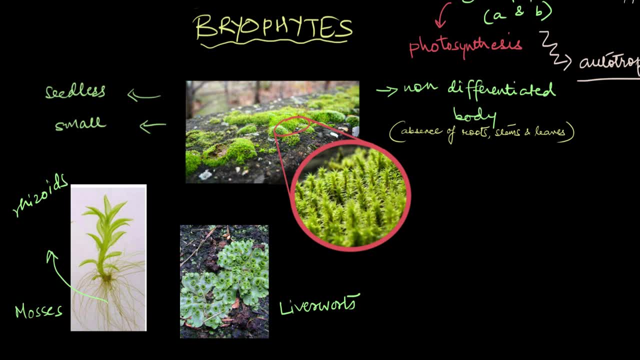 All bryophytes are so simple that they also completely lack vascular tissues. That means they have no xylem or phloem. But what do these tissues do again? Well, vascular tissues are specialized tissues that can conduct food and water to the entire. 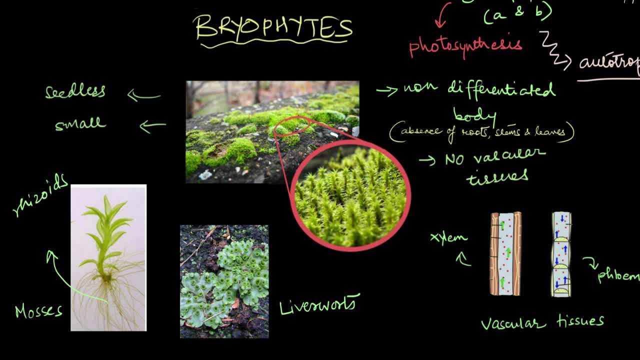 plant. Now bryophytes are so tiny that they don't really need this separate system of specialized tissues. They can transport these substances simply by diffusion or osmosis, But they can also conduct food and water to the entire plant. Now bryophytes are so tiny that they don't really need this separate system of specialized 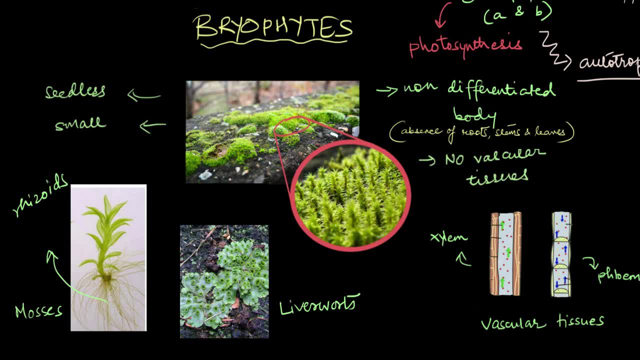 tissues. But the higher, bigger plants can't do that. For them, diffusion or osmosis aren't just enough, So they need this entire set, or this special set of tissues called vascular tissues, which is going to make sure that they transport the food and water to every part of the entire. 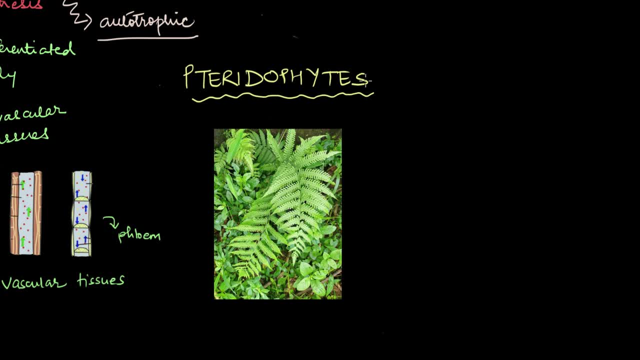 plant. Next in line are the pteridophytes, or division pteridophyta, which includes plants like ferns, horsetails, ground pines, etc. etc. Now, they are also very small. They are also seedless, just like the bryophytes, but unlike them, pteridophytes have vascular 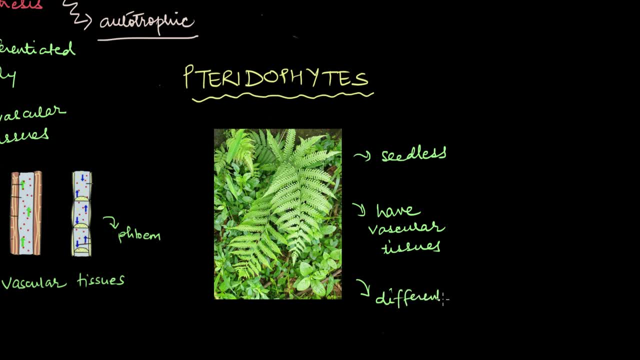 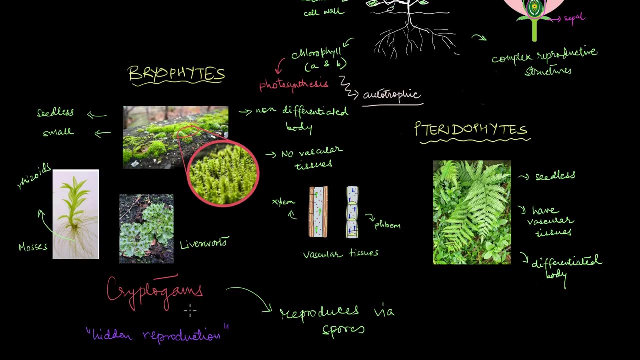 tissues. Moreover, their bodies are differentiated into roots, stems and leaves, and not just the lookalikes that we saw in bryophytes, but actual roots, stems and leaves, just like the higher plants. Both bryophytes and pteridophytes are often referred to as cryptogams. 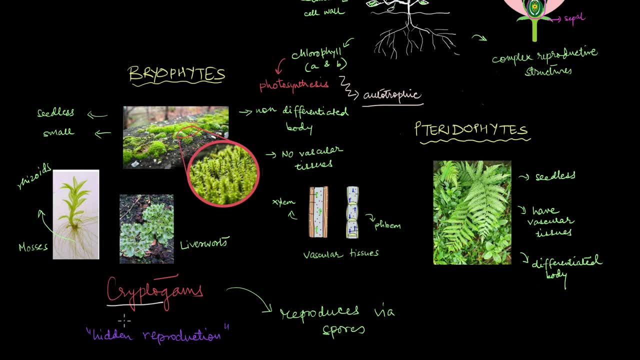 If you break this word down, crypto means hidden And gam, which comes from gamy, means to marry. So cryptogam roughly translates to hidden reproduction. But how is their reproduction hidden per se? Well, these plants, the bryophytes and the pteridophytes, they reproduce via spores. 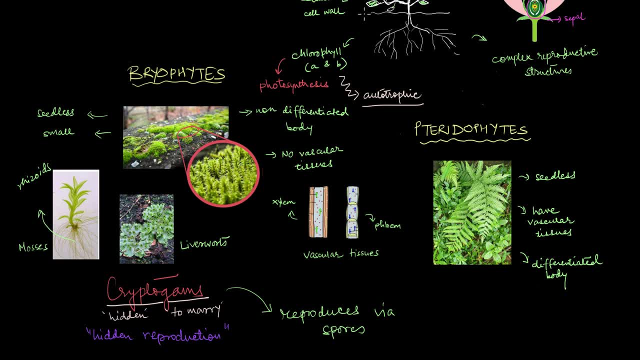 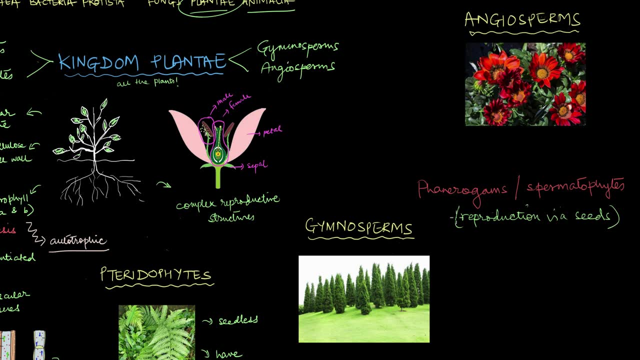 And spores aren't really something that we can see with our naked eye. On the other hand, the plants that reproduce via seeds are called Phenerogams or spermatophytes. Pheneros in Greek means visible, So Phenerogam roughly translates to visible reproduction, because we can see the seeds. 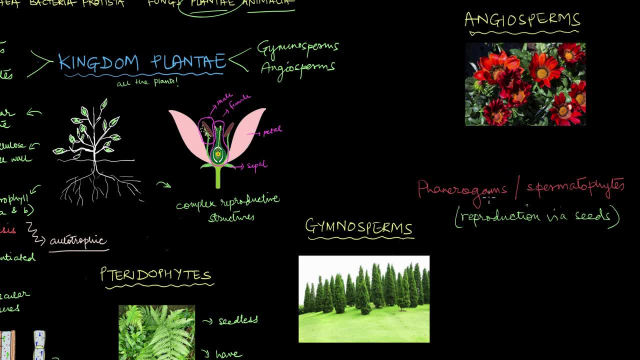 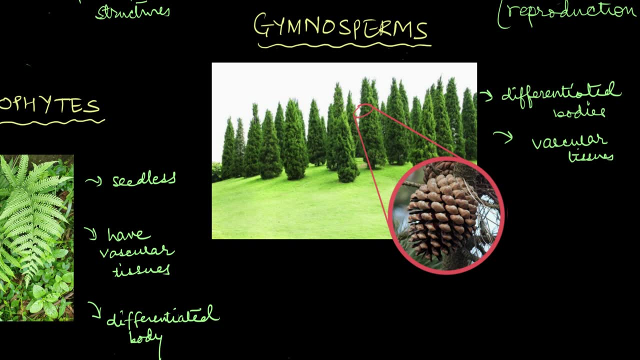 of a plant. Phenerogams or spermatophytes includes the gymnosperms and the angiosperms. Gymnosperms are more advanced than the pteridophytes. They have differentiated bodies, vascular tissues and, like we already know, they can.